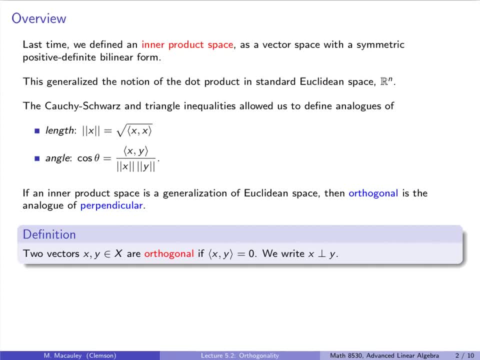 So two vectors are perpendicular in Euclidean space if their dot product is zero, And they are orthogonal in a generalized Euclidean space if their inner product is zero. We all know the famous Pythagorean theorem in Euclidean geometry, So here it is, in vector notation. 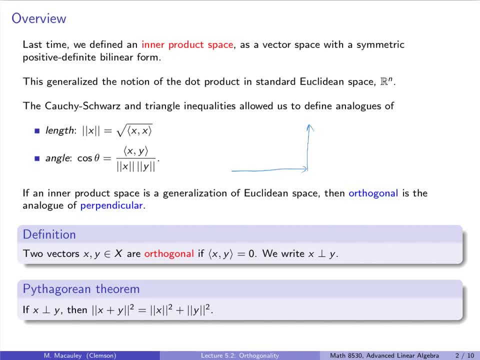 If we have two vectors, x and y, which are perpendicular, then that means they form a right angle, And so the hypotenuse is x plus y. So the Pythagorean theorem says that norm x squared plus norm y squared equals norm x plus y squared. 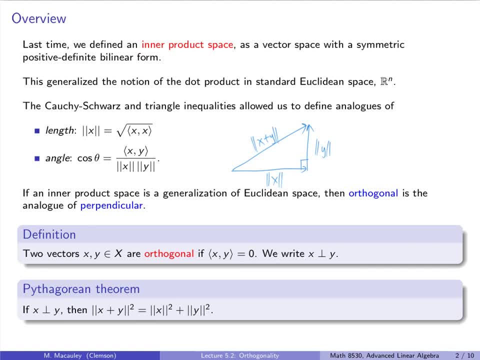 And this carries over exactly to general inner product spaces. And it's easy to see why. In the last lecture we computed that the norm of x plus y squared is the norm of x squared plus the norm of y squared plus 2x dot y. 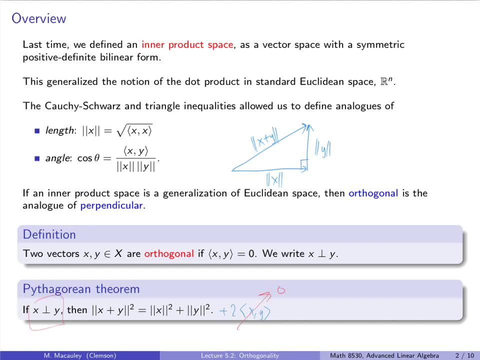 And if x and y are orthogonal, then that is just zero And we are left with the same old Pythagorean theorem. Now a word of warning. We saw in the previous lecture. I gave an example where the inner product of x and y 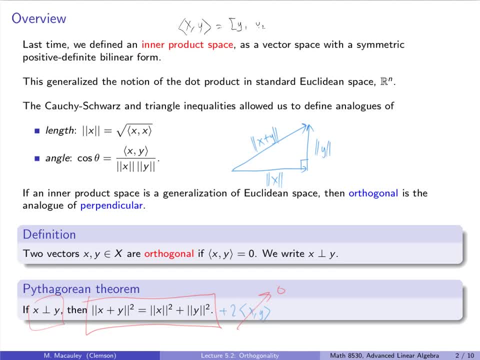 was defined by y1, y2 times 2, 1, 1, 2 times x1, x2.. And with this definition, the standard unit basis vectors are what we normally call the standard unit basis vectors: 1, 0 and 0, 1.. 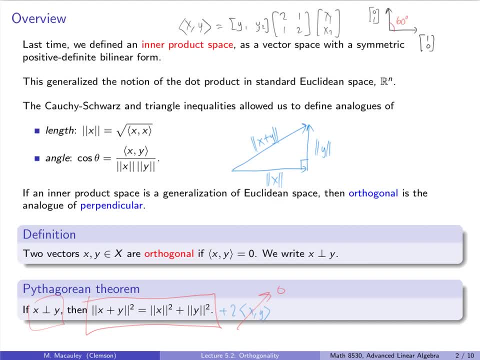 They ended up having only a 60 degree angle between them. So be careful when we say orthogonal, because how we embed these vectors using our standard coordinate system is not necessarily indicative of the actual coordinate system or the angle between them. So generalized inner products can be a little bit deceiving in this way. 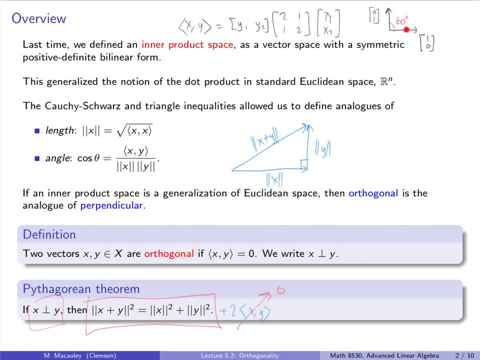 I think we also proved that these vectors had length root 2 with respect to this inner product, And I'm mentioning this here because we are going to come back to this example and we are going to figure out what vectors are orthogonal. It seems intuitive that I can ask what's orthogonal to 1, 0? 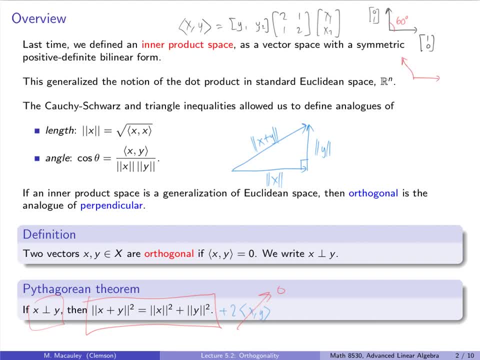 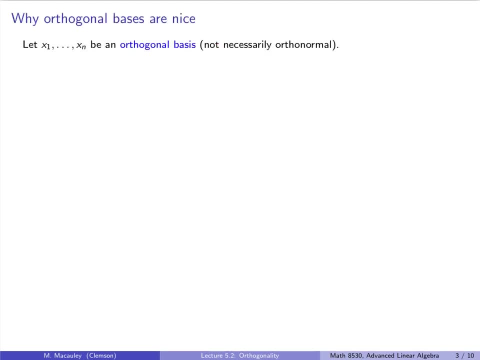 and it's going to be something out here. If this is 60 degrees, then 90 degrees is going to be something bigger than this, but the only question is how much bigger? To start off, I want to convince you why orthogonal bases are nice. 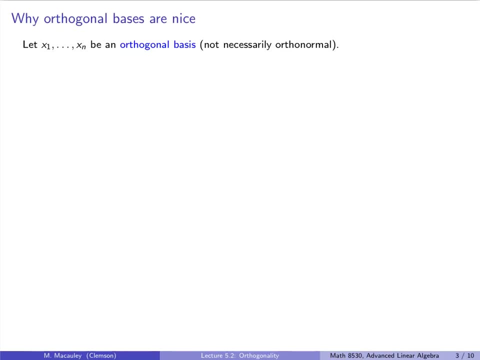 I mean, it seems obvious, but let's go through the motions. Suppose x1 up to xn is an orthogonal basis, not necessarily orthonormal. Now, I haven't defined orthonormal, but you likely know what it is and you might be thinking this, but all I'm saying is that these vectors 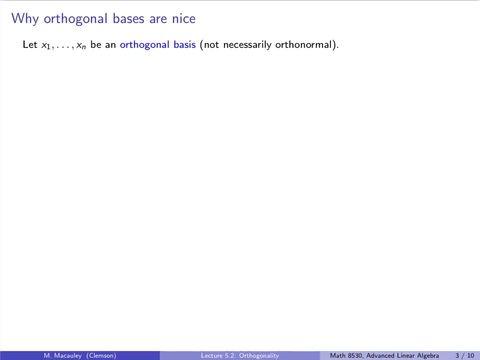 are mutually perpendicular. Given an arbitrary vector in x- because this is a basis- we can write v as a linear combination of the xi's. We can find a formula for ai by applying the following linear map to both sides. So let's take our inner product and let's plug in xi to the second coordinate. 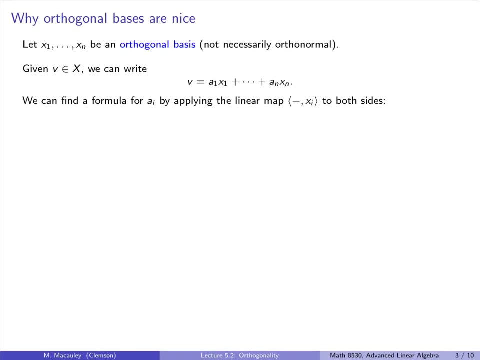 or the first coordinate, either one will work. Remember, if we do that to a bilinear function we get a linear function. So if we do that up here, then the left hand side becomes v, dot, xi. remember I still use the verb dot. 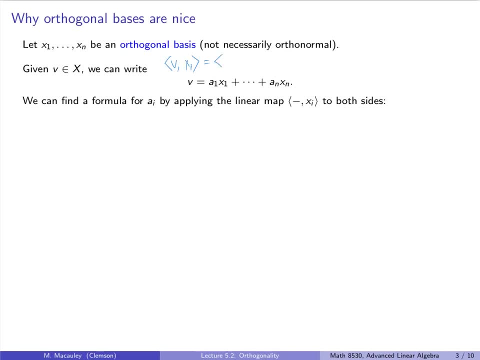 and the right hand side, we get a1, x1, xi, and I think you see what's going to happen: ai, xi, xi, dot, dot, dot, up to an xn xi, and the key is, because these are orthogonal, all of these terms are going to go to zero. 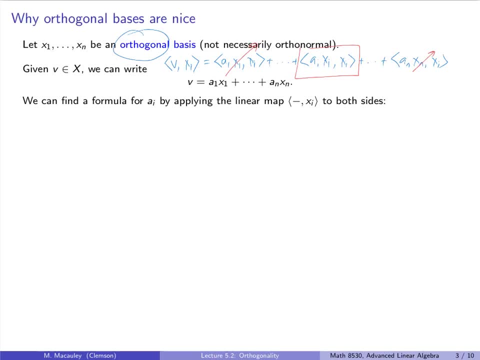 except for the ith one, and of course, an ai is going to pull out, and what we get is that v dot xi equals ai times xi dot xi, and this gives us a formula for ai, Namely, ai is the inner product of v and xi. 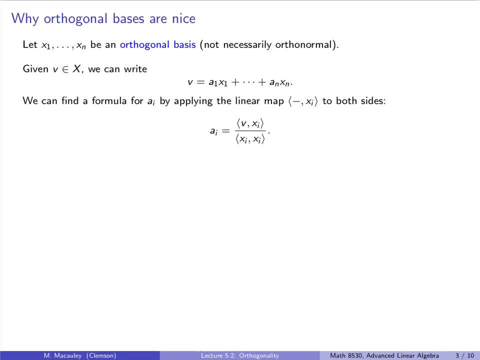 with the inner product of xi in itself. What we are basically doing here is projecting the vector v onto the ith coordinate xi. So ai is the magnitude of v in the xi direction. A magnitude is length, and for that we need an inner product. 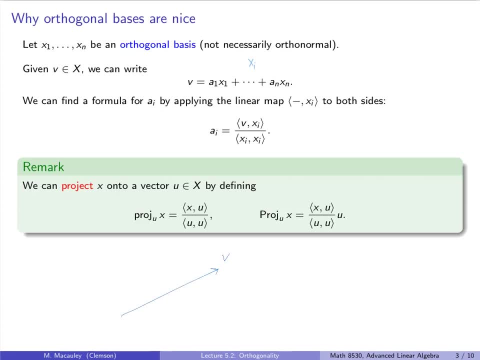 So a way to think about this pictorially is: if this is v and this is x1,, then this length here is: how do I want to draw this? this length here is ai, and we also may want to speak of the vector. 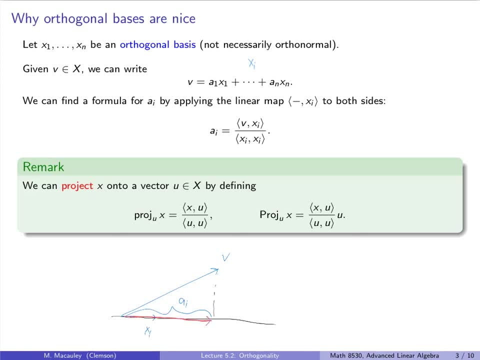 in the xi direction of magnitude ai and in other words ai, xi, and so v is a1, x1 plus ai xi plus an xn. So this is the component of that vector, v in the xi direction. So I will give a definition and notation for this. 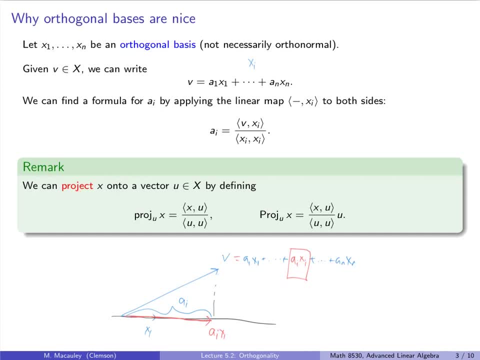 sort of a remark, sort of a definition: The projection of a vector x onto another vector u. so there's two things you want to keep track of, both the magnitude, and I will denote that with a lower case projection: x dot u over u dot u. 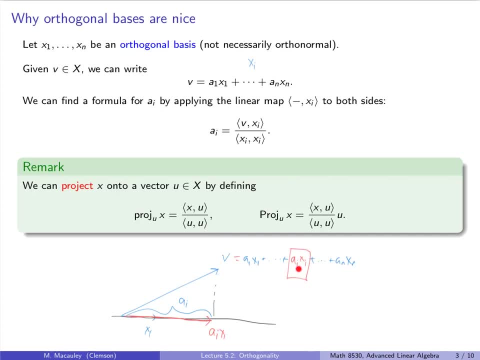 and then also the vector, so that component ai xi. well, I guess in this case it's an x and a u, so that I'm going to write that with a capital P projection of x onto u, And that brings us to a new definition. 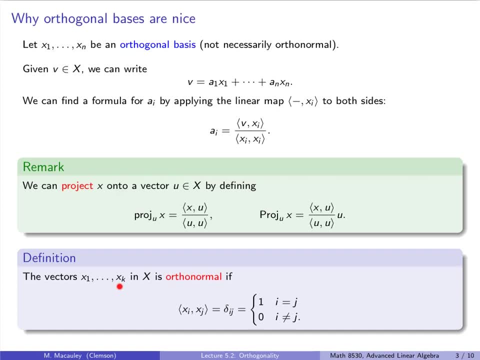 We have vectors. we have vectors x1 up to xk which are orthonormal. if you take the inner product of any two of them, you get zero if they're different and one if they're the same. So this part means that they are mutually orthogonal. 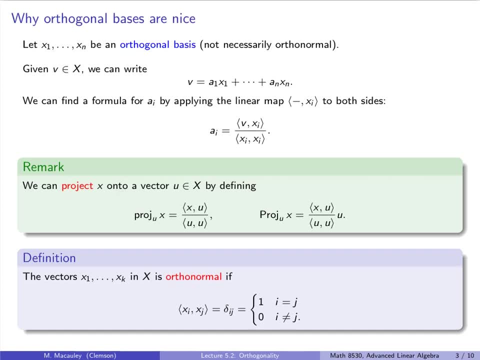 and then the other part means that each one has unit length. So remember that the norm of xi squared is xi dot xi, and we want each of these to have length one. So sometimes we denote this with delta ij. so this is the Kronecker delta. 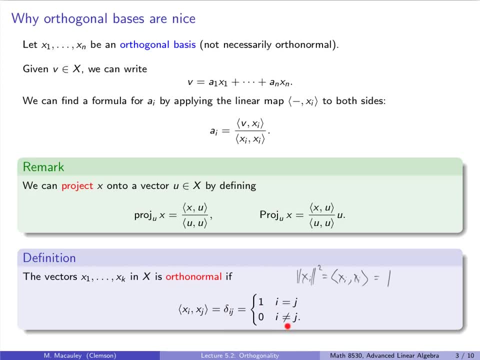 so this is one if i and j are the same and zero otherwise. So a way to think about this, how I visualize this, is: I think of this as, like our standard unit basis vectors, where everything is at right angle. I've already given you the warning that sometimes the vectors 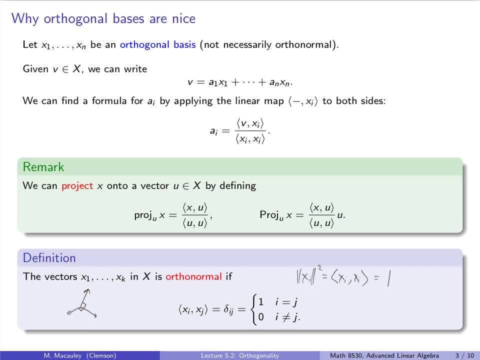 in different inner product spaces may look how we render them, draw them to be 90 degrees apart, but the actual angle is like 60. So I've given you that warning. I don't need to go over that again. This is the mental picture I have for orthonormal vectors. 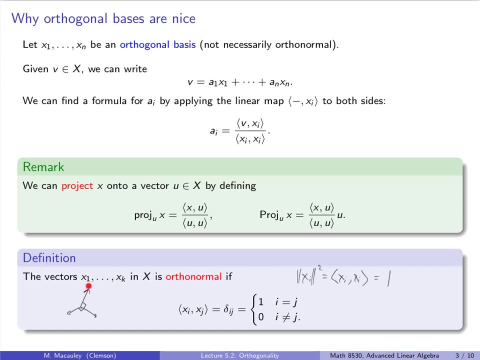 And we're not assuming here that we have n vectors, so this doesn't necessarily have to be a basis. But one comment about this is: when we have an orthonormal basis, these projections become a lot simpler, So in that case we can just ignore the bottom of that. 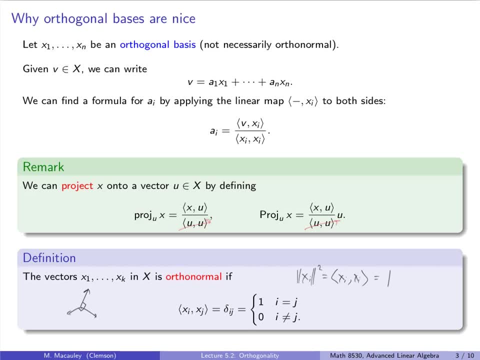 because that's equal to 1.. So let me give you a simple example. I might have done this in an earlier lecture. I really don't remember. I know I've done it in at least one or more of my other classes. So let's take a vector. 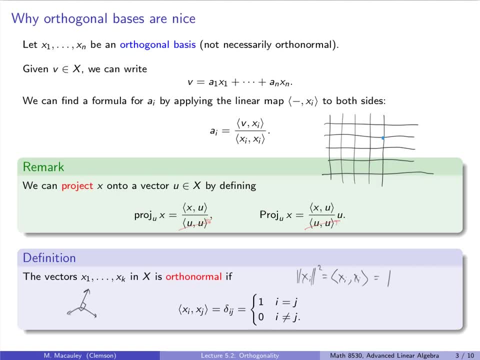 I'm going to say so. that's this vector, right here. v and this is, which, of course, is 4e1 plus 3e2.. And e1 is down here. this is we're going to use the standard dot product. 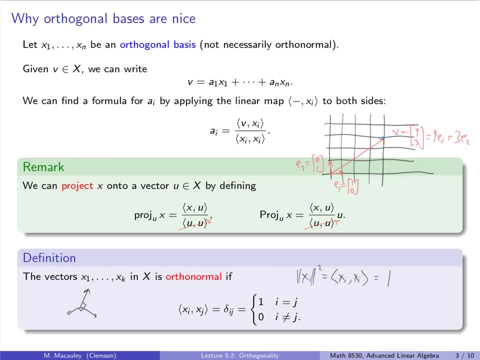 e2 is. Now I can ask: suppose this is like your velocity vector. I can say: how fast are you traveling in the x direction? And the answer is 4.. You just drop a perpendicular and it's this length, right here. 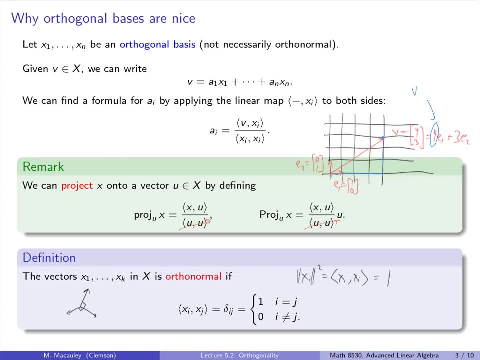 So that is 4, and that is ve1,. and how fast are you traveling in the y direction? That's going to be 3,, that's ve2.. Now another question I can ask is: how fast are you traveling in the northeast direction? 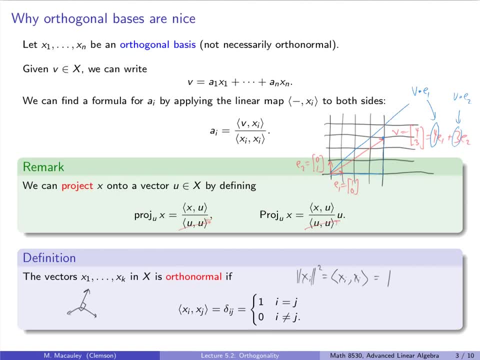 So that's in this direction, and the answer to that is: you take the standard unit basis vector here, and I'm going to call that v1, which is root 2 over 2,, root 2 over 2, and you project v onto v1,. 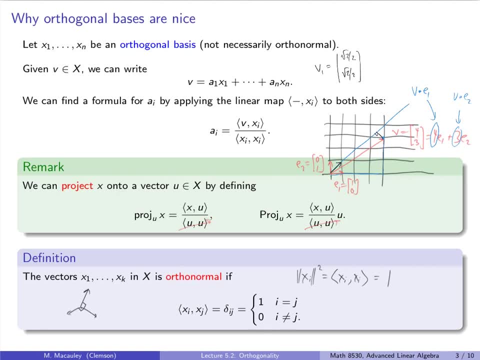 and so I should say: this is ve1, is this dot for 3,- the order doesn't matter- symmetric, and this is approximately this 4.9.. And so that makes sense that this vector is length 4.95. in that direction. 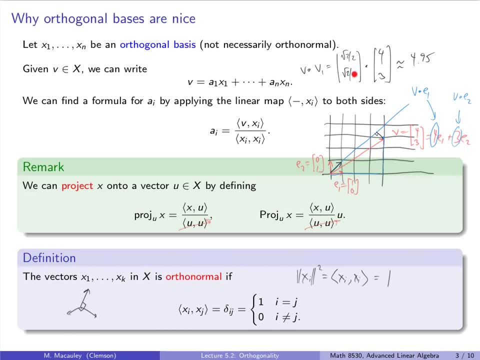 Now what's often the case? you don't necessarily have an orthonormal basis, and I'm going to do some examples later in this lecture, especially involving functions and polynomials, where we don't necessarily want to normalize the vector at every step. 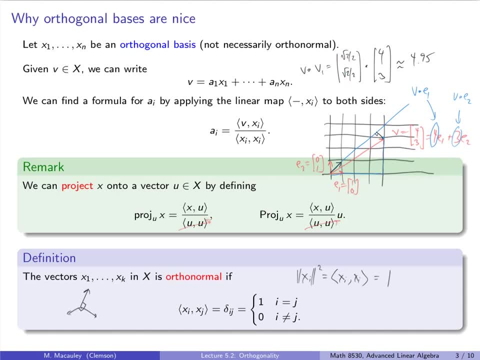 because we'll get nasty radicals. So if instead we just had the vector here, v1 here? so I'm going to say I don't know what letter to use. say u is equal to, in this case, 1,1,. 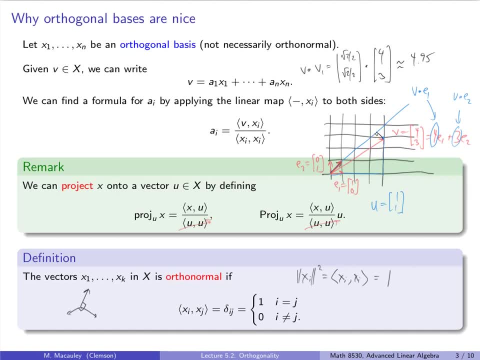 and I want it to project v onto the u direction, then I use this full formula, or either one of these full formulas, depending on whether we want magnitude or the vector, and I will say so: v dot u. I'm going to switch to this inner product notation. 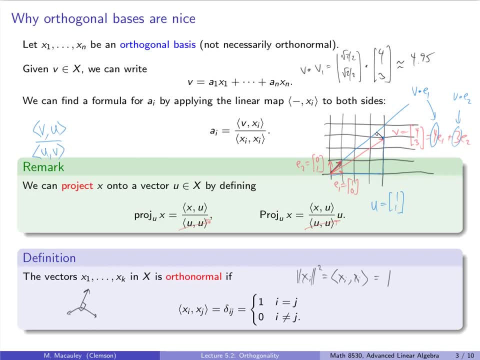 u dot u actually. let me do it this way: we can normalize u first, so we can project v onto the. so the normalized version of u is u divided by the norm of u, so that is the projection onto the unit basis vector in the u direction. 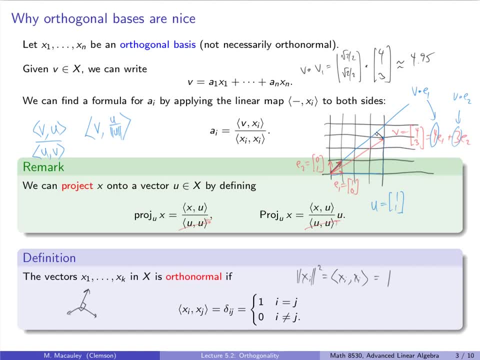 and then this vector, that unit vector again, is u over norm u. So in this case we can write this as v dot u divided by norm u squared, and this is v dot u over u dot u. So this is another way to derive. 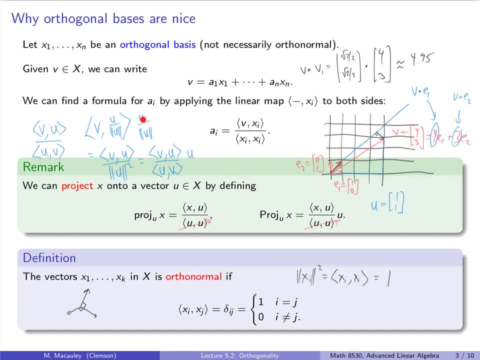 oh, and then there's a u here that doesn't go away, So I also forgot my u right here. But this is another way to re-derive this projection formula, in addition to what we did up here, which was just taking the. 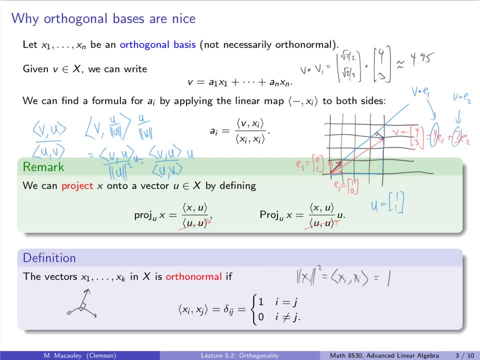 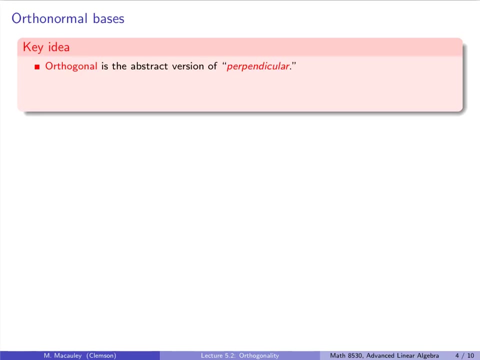 applying this linear map to both sides, So I hope this helps. this is what we're doing. sometimes we have unit vectors to project onto, other times we don't, so we use this more complicated formula. To summarize: so far, orthogonal is the abstract version of perpendicular. 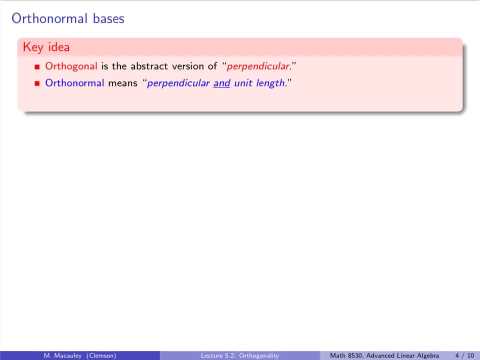 and orthonormal. orthonormal is the analog of being perpendicular and unit length. Orthonormal bases are really desirable If x1 up to xn is an orthonormal basis and we have two vectors in our space, say x and y. 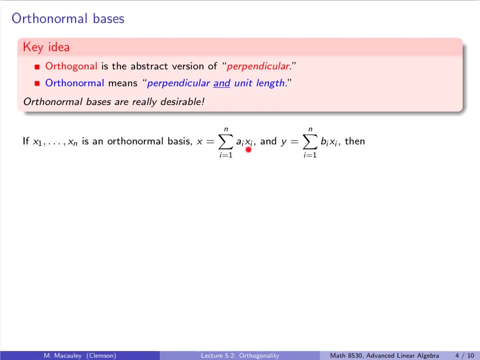 let's write x as a sum of ai, xi and y as the sum of bi- xi. then, as we just saw, ai is the projection of x onto xi or the inner product of x with xi. We can keep going with this idea. 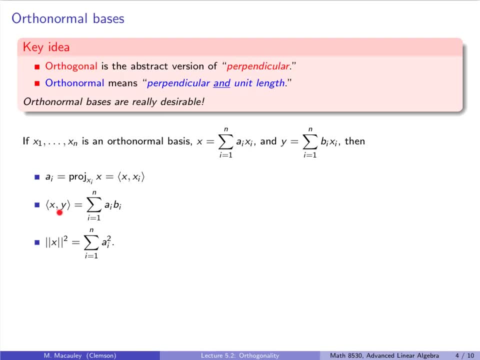 and I claim that the inner product of x and y is just the product of ai times bi from 1 up to n. Now you may look at this and say: wait, this is just the standard dot product and our inner product is not necessarily the standard dot product. 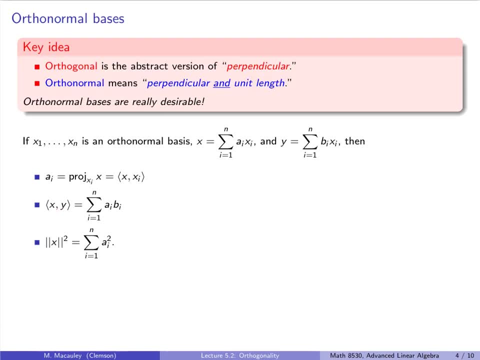 and both of those are true. So our standard inner product might be: let's do that example that we did before: b1, b2, times 2, 1, 1, 2, times a1, a2,. 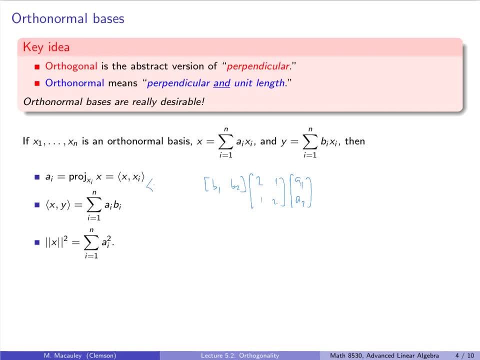 so we're here and we'll do this example fairly soon as well. the inner product of x and y is- I'm going to write this as y transpose ax, even something like this- that's definitely not the dot product if we take an orthonormal basis. 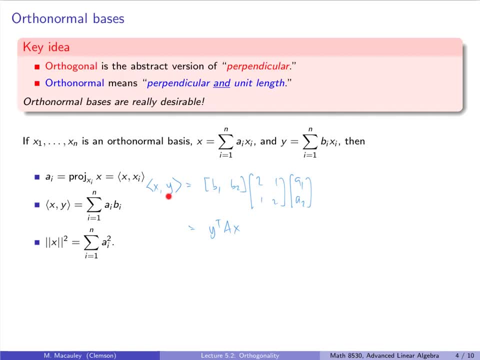 with respect to this inner product. Now, remember, that's not going to look like a standard, orthonormal basis with respect to the dot product. It's going to be as we will see shortly. it's going to look something like a vector here and a vector out there. 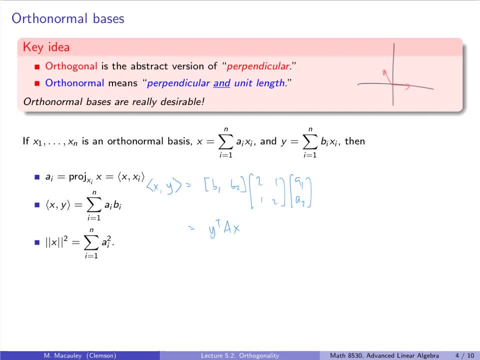 But if we take one of these orthonormal bases, then with respect to that basis, the inner product of x and y behaves or computes just like the dot product. Now let's see why that is So: the inner product of x and y. 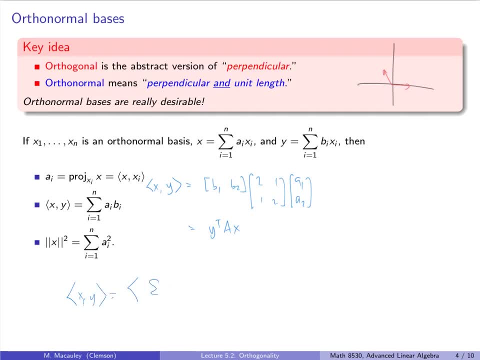 is the inner product of aixi. it's just bilinearity and orthogonality bixi, so we could break this up into a giant sum. so this is: i equals 1 up to n. i equals 1 up to n. 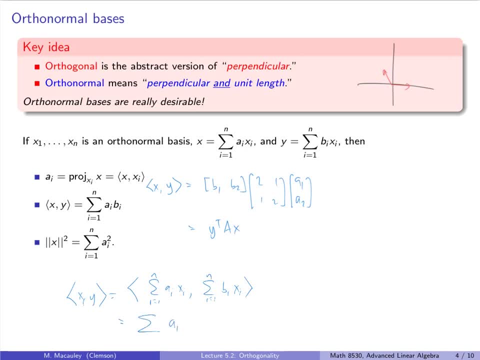 so we break this up into a giant sum of aixi, bj, xj, over all i and j, so you can think of this as a double sum if you want. and of course all of these terms are going to be zero, except for the ones where i and j match. 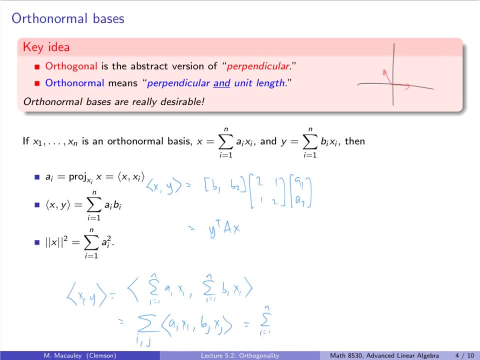 So we get i equals 1 up to n of aixi bj, xj, and that's just the sum from. i equals 1 up to n of aibi xi, xi. this, of course, is just 1, so we get this sum as desired. 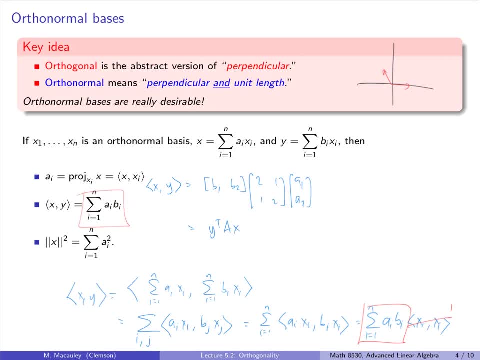 So at first glance it's a little bit counterintuitive. but the big theme here is: if we pick an orthonormal basis, any inner product basically behaves just like the dot product. And of course, a special case of that if we take y to be equal to x. 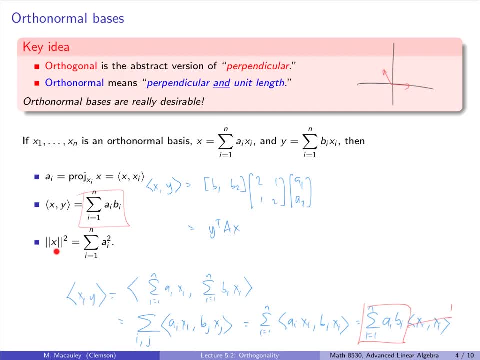 is that the norm of x squared is just the sum from i equals 1 up to n of ai squared. So this should look just like the Pythagorean theorem, but in a general inner product space. So that is why orthonormal bases are really desirable. 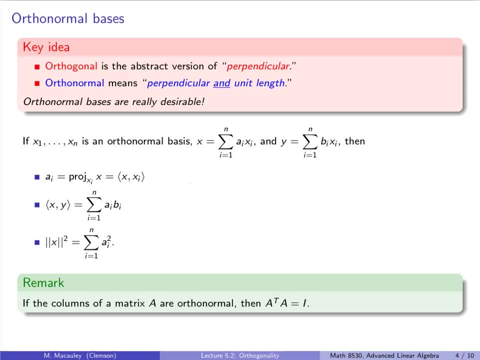 One last comment that I want to make here, because it will come up a number of times in the future, is that if we have a matrix A and the columns are orthonormal, then they're automatically an orthonormal basis. so say x1,, x2, up to xn. 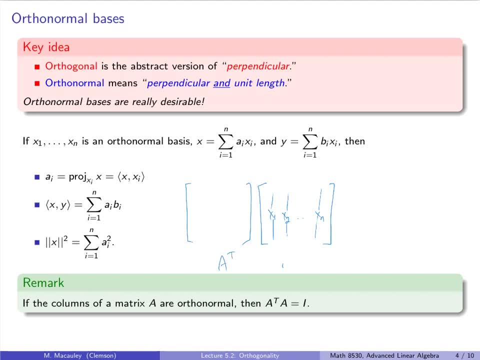 and we take A transpose. A think about what that looks like. so A transpose, the rows are going to be an orthonormal basis, then this is going to, then the entries are going to be. so this first entry is going to be. 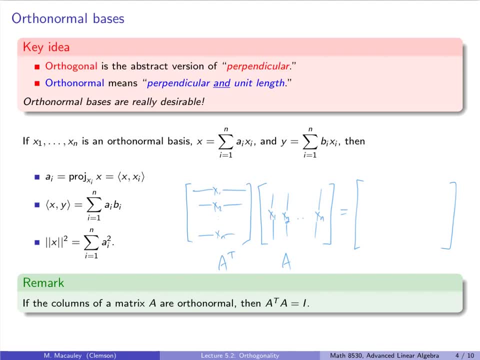 x1 dot x1,. so here I'm going to use just the standard dot. well, I'll use inner product notation. why not x1 dot x1,. and then the next one is going to be x1 dot x2,. 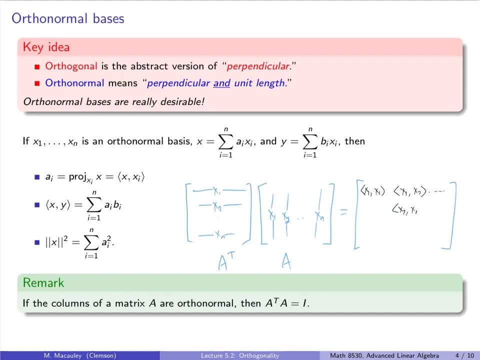 etc. x2, dot, xn, x2, so this matrix is the identity. I should say: what does it mean for this matrix to be the identity? Well, that happens if, and only if, all of these diagonal entries are 0, in other words, 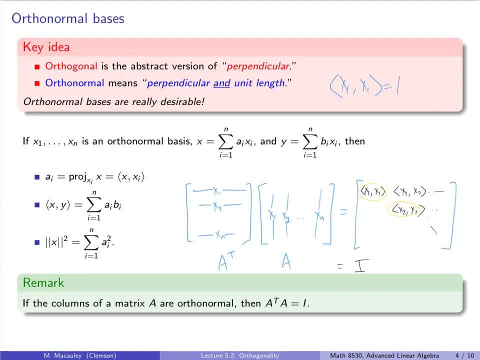 if xi dot xi equals 1, and if all off-diagonal entries, xi dot xj equals 0, so that is equivalent to the columns of the matrix being orthonormal. so that will come up later. unfortunately, such a matrix is. 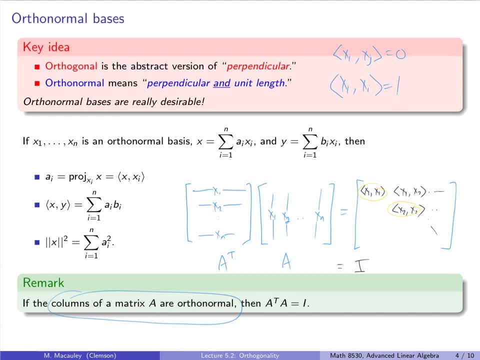 not said to be orthonormal, but it's said to be orthogonal. so an orthogonal matrix has orthonormal columns. I think that's a terrible definition, but it is what it is. we have to live with it. Let's now do some examples. 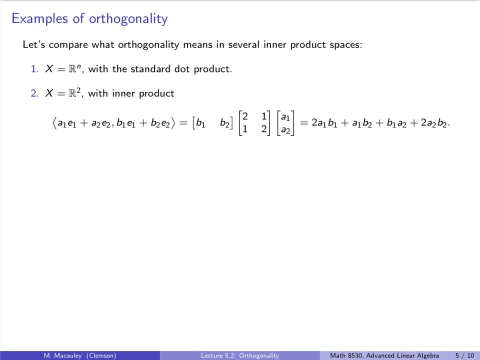 of orthogonality. so let's compare what it means in several inner product spaces. Now we know what it means in Rn with the standard dot product. let me just draw R2 here. E1 and E2 are of course orthogonal. 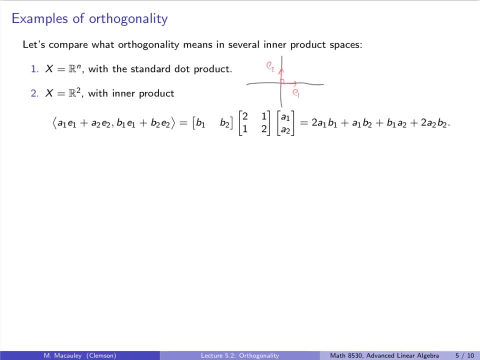 because their dot product is 0, and we saw in the previous lecture that these are not, or that the angle between these two was 60 degrees and with respect to this curious inner product. so let's go back and review that and take it a little bit further. 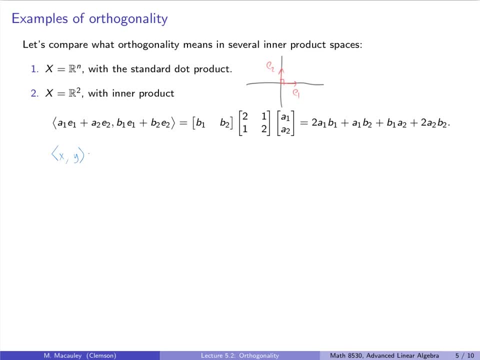 so here the inner product of X and Y. let me write X as A1, A2, and Y as B1, B2,. this is defined as Y. transpose AX. Now let me draw the same picture again. so if E1 is this vector: 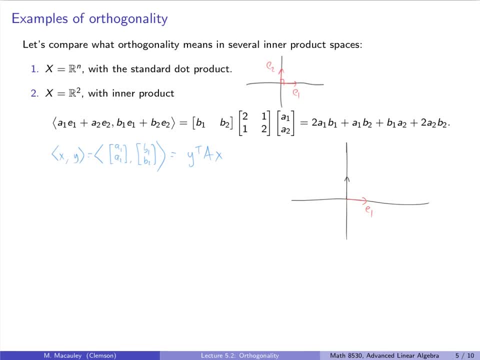 and then E2 is up here. I'm drawing it in black because it's not really the vector I want to highlight. then we can ask what this angle is, and in the previous lecture we determined that the cosine of that angle, which we know, is E1, dot, E2,. 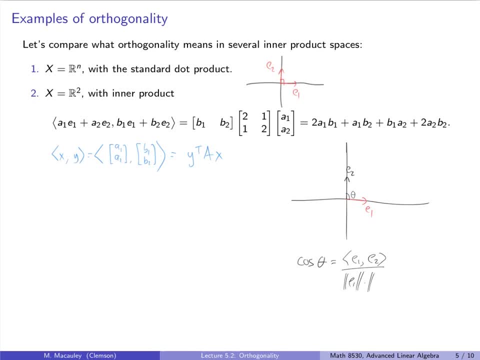 divided by the norm of E1 times the norm of E2, and we computed that E1 dot E2 was just 1, and each of these was root 2,- perhaps surprisingly with respect to this strange inner product. so this is equal to 1: 1⁄2. 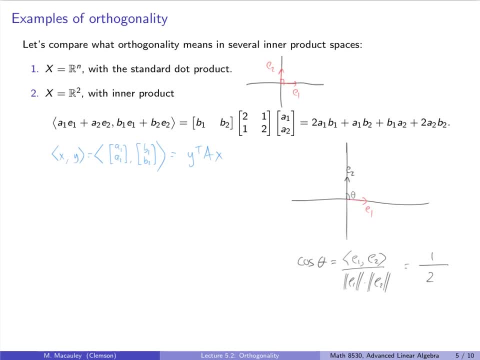 So in standard Euclidean space the angle of 60 degrees has cosine 1 1⁄2, so even though these things look to be perpendicular with respect to this strange inner product, they really are to meet at an angle of 60 degrees. 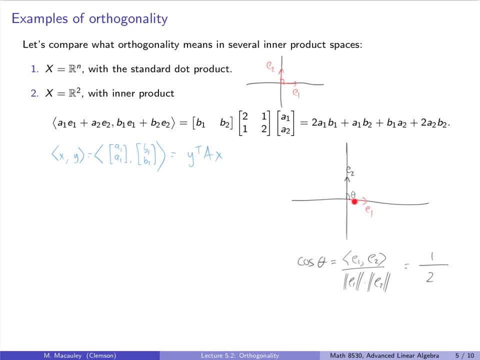 So that begs the question: what vector is perpendicular or orthogonal to E1?? It would make sense that it's going to be something that is out here, but what is that vector? So let's solve for that. Let's put E1 in for x and solve for y. 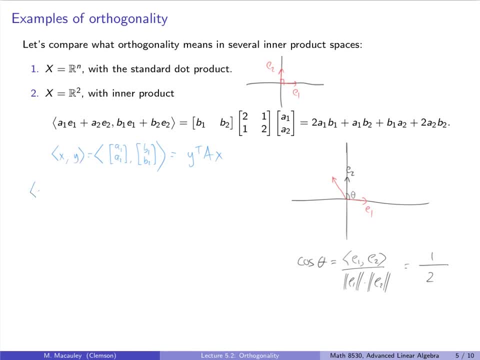 So E1 dot y is b1, b2, 2, 1, 1, 2 times 1, 0, and this is b1- b2, b2 times 2: 1, and this is 2: b1 plus b2 equals 0.. 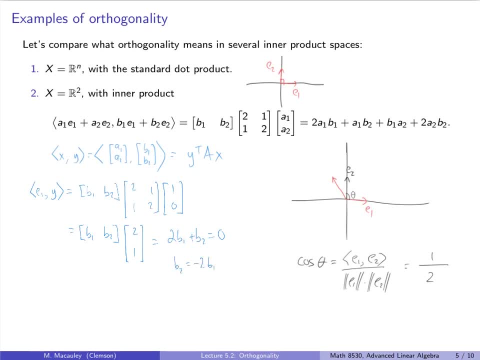 So, in other words, b2 equals negative 2, b1.. So that means that this entry is negative 2 times, whatever that entry is. So, for example, the vector negative 1, 2, I don't know what I want to call this. 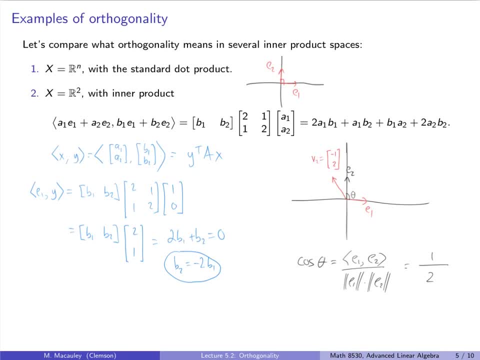 let's call this v2, this is orthogonal with E1. So this may be a little bit counterintuitive, because it looks like the angle is more than 90, but it's because it's with respect to a different geometry. Now, something also a little bit strange is 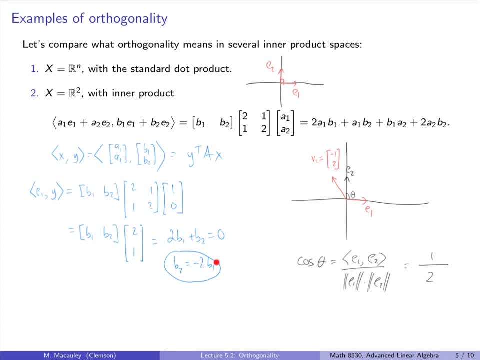 I said, b2 is. so anything, that's any vector that satisfies this, is orthogonal with E1, and well, you know what else satisfies that Down here? if you take the vector 1, negative 2, these things are: 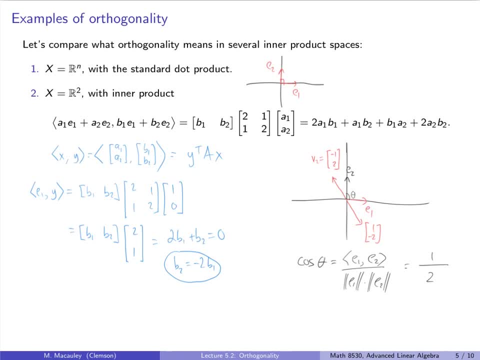 this is also orthogonal to that, by the same reason, because it satisfies this equation. So, yeah, perhaps strangely, this angle here is you can think of it as like 90 degrees. well, and when I say, you think of it as 90 degrees. 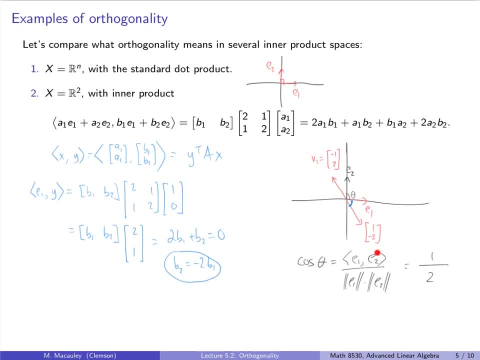 I mean the cosine of this is 0,, because the cosine of that angle is E1. dot this thing which divided by the norm, which is 0, and this is analog of a right angle up here as well. I will leave it as an exercise. 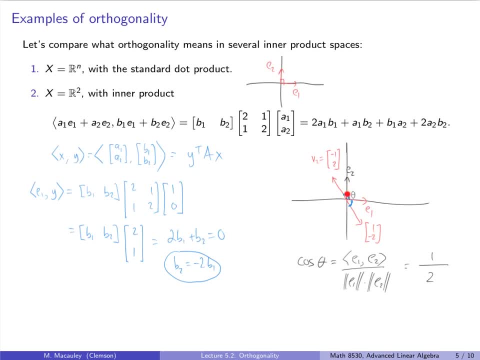 to figure out what is orthogonal to E2.. It shouldn't be much different than this in terms of the process. it just comes down to plugging in the numbers and figuring it out. Next, for fun, I'll give you a quick high level tour. 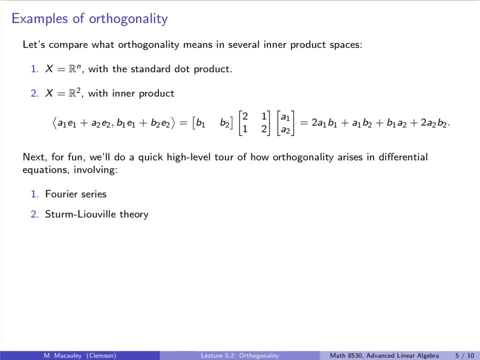 of how orthogonality arises in differential equations and related topics, In particular Fourier series and Strum-Liouville theory. So I'm not going to give a lot of details, especially because these all involve infinite dimensional vector spaces and when you have something like that, 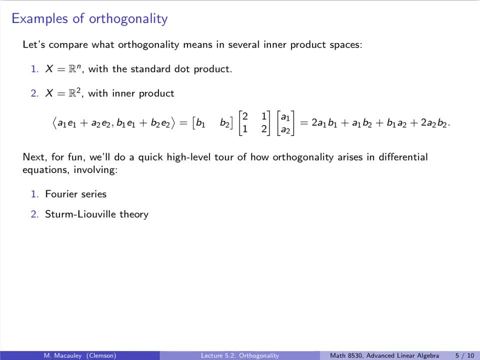 you have a big issue about convergence and infinite sums, and what does it mean to converge in norm or converge pointwise, things like that? So I won't get into that, but I just want to give you the flavor of why orthogonality is important. 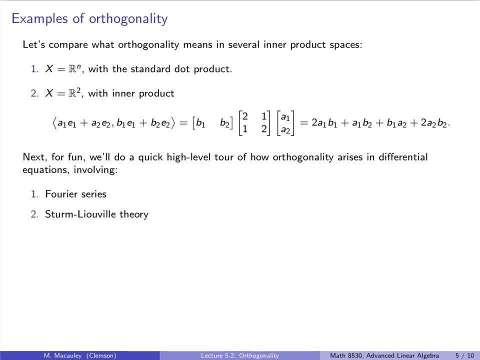 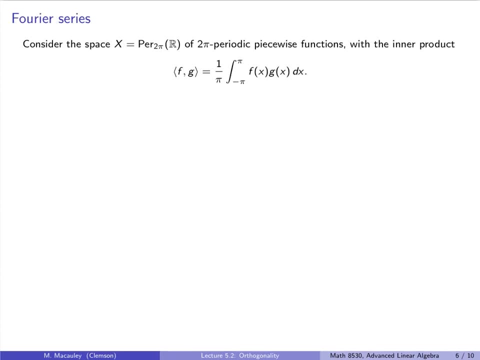 beyond just things like Rn with the standard dot product or with some weird little inner product like this. Our first example involves Fourier series. for this let x be the space of 2 pi periodic, piecewise real valued functions and define the inner product between f and g. 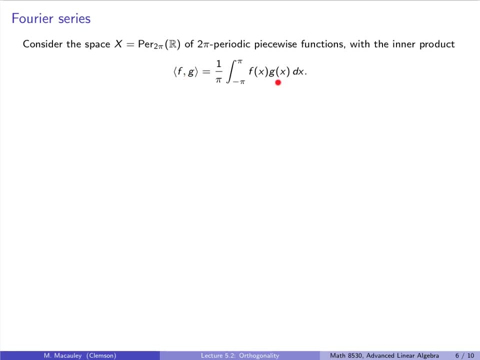 as the integral of f of x times g of x, from negative pi to pi divided by x. So the integral is, like the analog, the continuous version of the sum. so for the dot product, we multiply, we multiply the coordinates together and add them up. 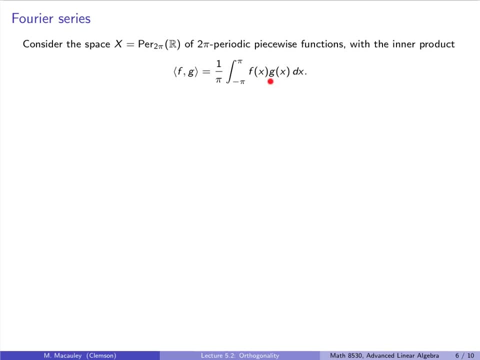 and here we're multiplying the individual points at every x, f times g, and adding them up over one complete cycle. Now, before I go further, let me say a couple of comments. First of all, 2 pi. periodic I don't necessarily mean the period is exactly 2 pi. 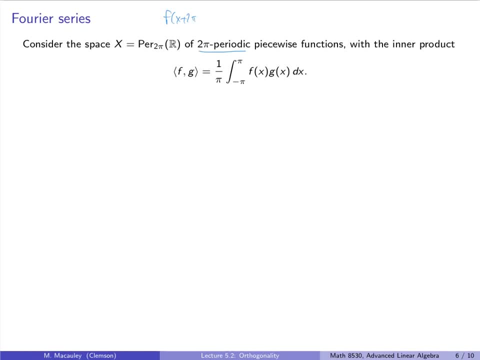 I just mean that f of x plus 2 pi equals f of x for all x, So maybe the period is pi or maybe it's pi over 5.. I just mean that after 2 pi the function has cycled some integer number of times. 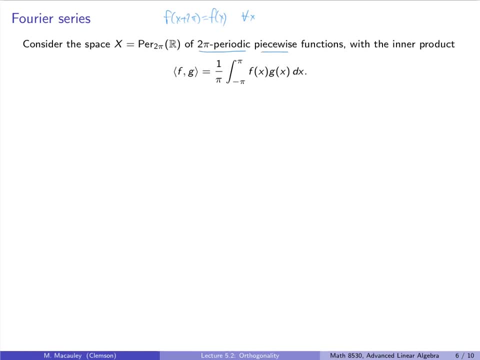 Now piecewise. I don't need to restrict these functions to be continuous, but I need. I just need them to be integral. but not any integral function is going to work. So, for example, here's a non, here's one that won't work. 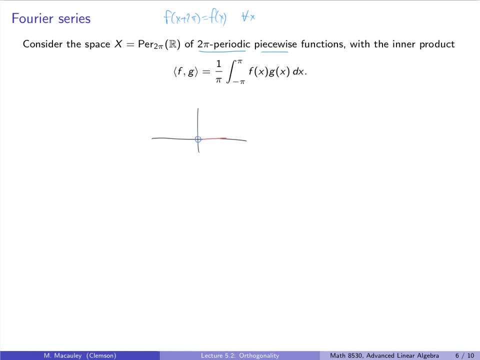 So if you have the function, let me use red. it comes out a little bit better. That is 0,. so on negative pi to pi, it's 0 everywhere, except maybe it's 1 at the origin. So if we were to repeat this function, 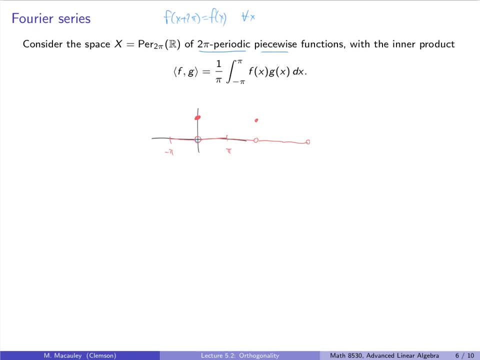 in other words make this periodic and then compute the inner product of this or I guess, the the norm of this function. Let's just do the norm squared, because that's easier. So that's the inner product of f with itself, That's 1 over pi. 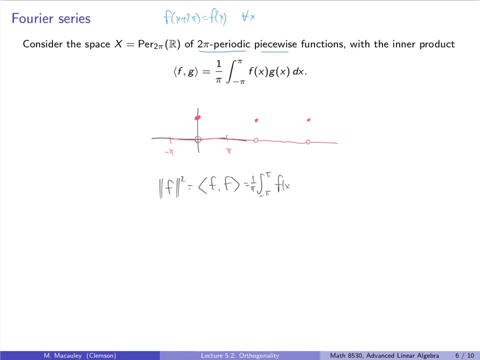 negative pi to pi. f of x squared dx, We're going to get 0, because if we integrate this function, it's 0 almost everywhere, everywhere except this one point. So the integral of that function is 0.. But if we include a function like this: 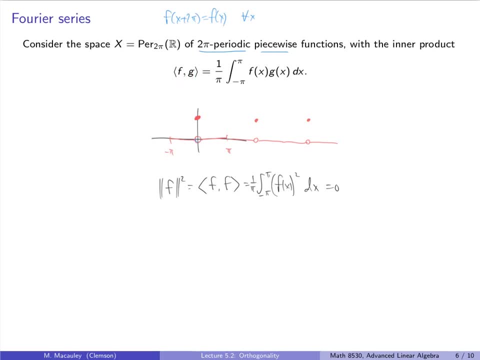 then this inner product is not going to be positive, definite. So that's why I say piecewise, and we don't need them to be continuous, And actually what we'll do is we'll talk about how. so the idea of a Fourier series. 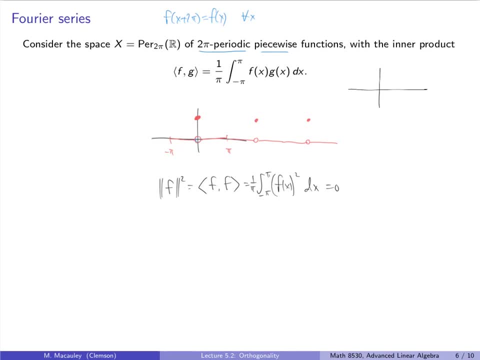 is that we can write periodic functions with sines and cosines, And that includes discontinuous functions like square waves, So we definitely want to include these in our space. I claim that the set of all cosine of x and sine of mx. 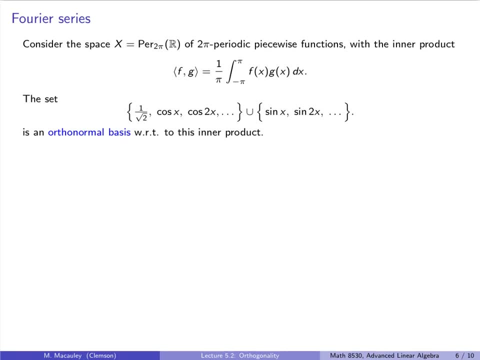 is orthonormal with respect to this inner product. I'll get to this weird constant in a moment, But first let me just verify that the sines and the cosines are orthonormal. What that means is that the integral. well, I write it as an inner product first. 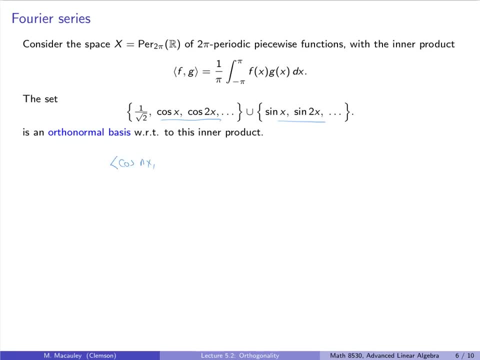 That means that if I take any cosine of nx and I take the inner product with the sine of mx, I'm going to get 0. So by definition that is 1 over pi negative pi to pi cosine of nx, sine of mx dx. 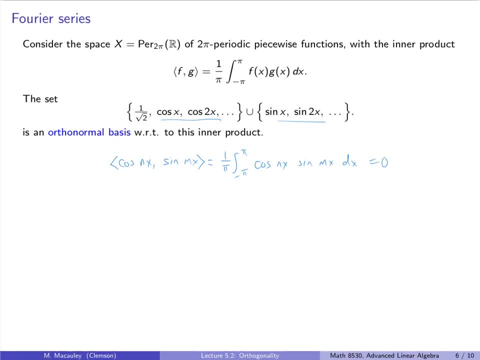 and I claim that that's going to be 0.. Similarly, if I take the cosine of nx and the cosine of mx, that inner product, that's going to, by definition, 1 over pi negative pi to pi. cosine of nx. 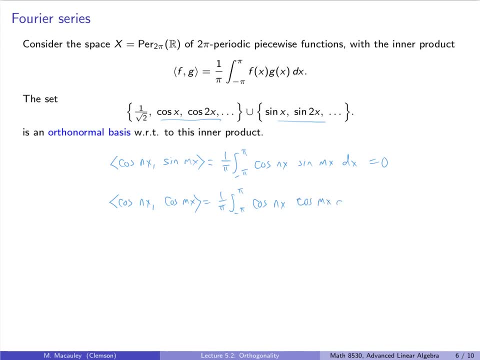 cosine of mx dx that this is going to be the Kronecker delta nm. In other words, this is going to be 1 if n equals m and 0 if n is not equal to m, And this is something you can easily check. 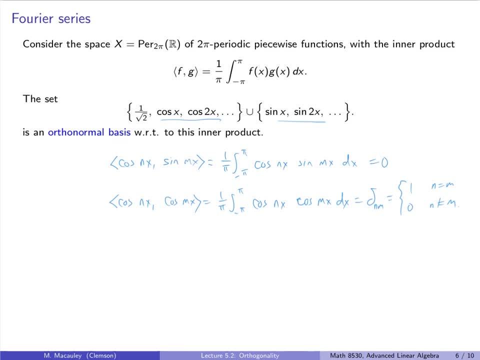 with trick identities. or I think probably the easiest way is to write cosine, as I'm going to write it like: cosine of x is e to the i? nx plus e to the negative i? nx over 2, and sine of x equals e to the i? nx. 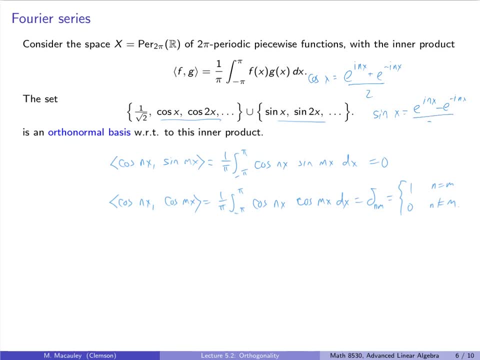 minus e to the negative i, nx divided by 2i, So that it's easy to check these identities hold. and there's actually one more that we need. We need that, the sine of nx, sine of mx, or that integral. 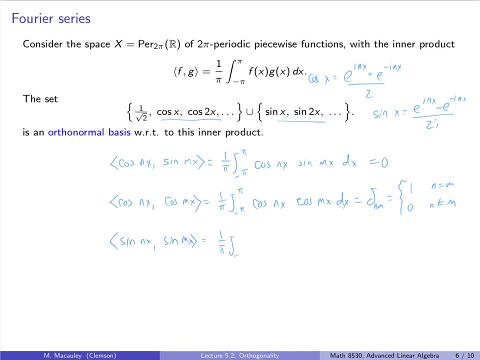 is, which it is 1 over pi times negative pi to pi, sine of nx, sine of mx dx, that this is also equal to delta nm as well. So if we can prove, if we verify all of these things, then this set of sines and cosines, 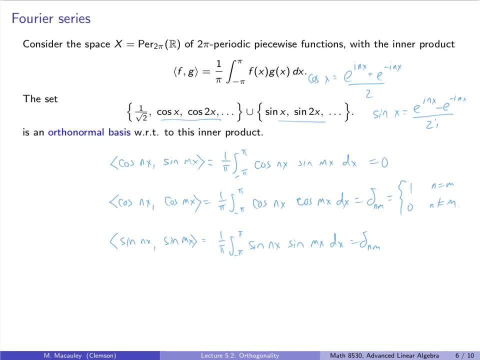 is indeed orthonormal. Now this last function. it's slightly unfortunate, I guess, that if you compute the norm of the function 1, or let's compute the norm squared, that's 1 dot 1, which is 1 over pi times negative pi to pi. 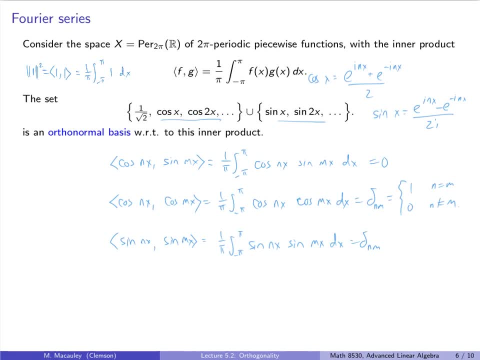 times the function 1, times dx, And this is easily seen to be to be 2.. So unfortunately, the norm of 1 is root 2.. So if you want to normalize the constant function, you write it as 1 divided by root 2.. 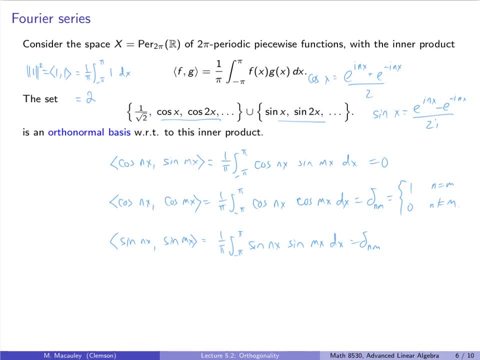 And now this thing has unit length And it's also easy to check that- that if you take the inner product of cosine of nx and 1, that you're going to get 0. And similarly, sine of nx with 1 is going to give you 0 as well. 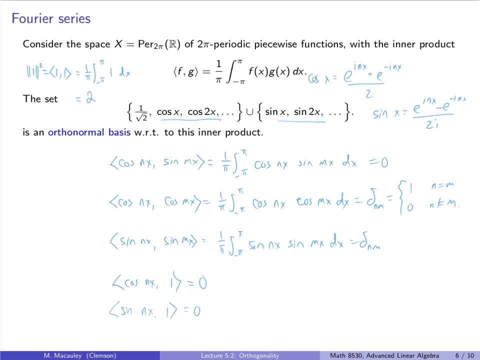 for any scalar of 1.. So these are orthogonal. And if you normalize this they become orthonormal. And this is easy to see, because what is this inner product? It's just the integral of cosine of nx, over from negative pi to pi. 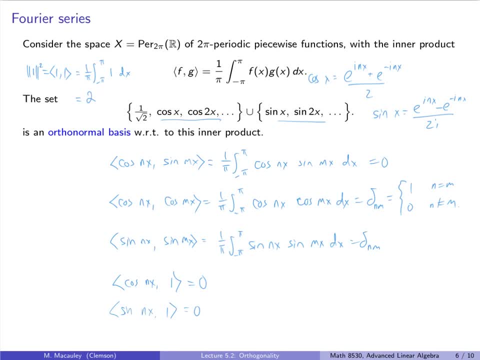 And think about a side area, you're going to get 0.. Now I guess one thing I didn't justify is: why is this actually a basis? So it's a non-trivial fact that every function in this space can actually be written. 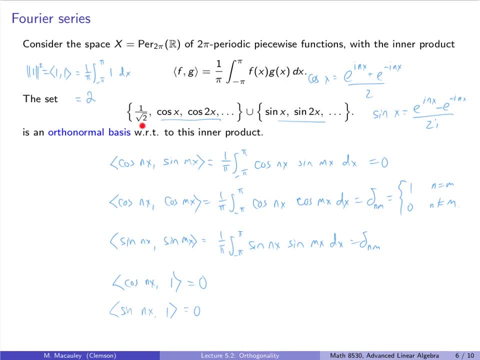 using sines and cosines and a constant. Now any audio engineer or musician is going to tell you that and say, well, yeah, it's just a sound wave and it breaks up into its fundamental components, So I'm not going to prove that. 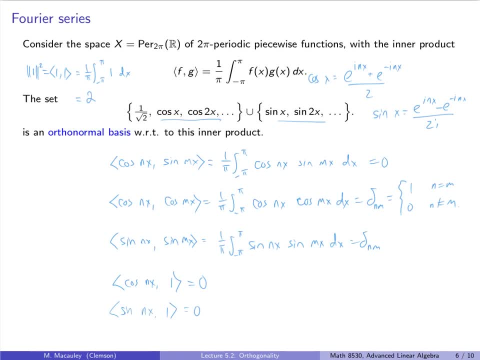 but I will claim that this is indeed not just an orthonormal set, but an orthonormal basis. What this means is that we can write each 2 pi periodic function uniquely as a linear combination of these sine and cosine waves and a constant. 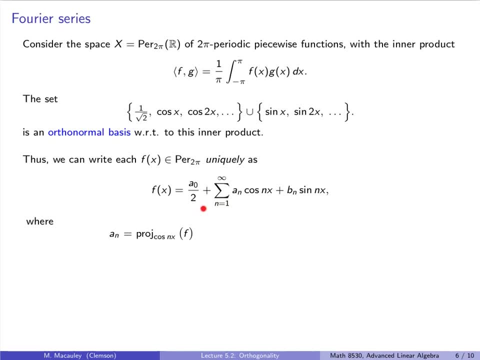 Now, the fact that I'm writing this as an infinite sum is one of those details that I'm again I'm sweeping under the rug. It's beyond the scope of this class, But it is necessary if we want to write functions like a square wave. 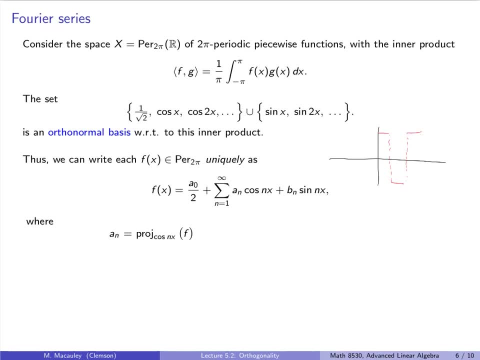 which is discontinuous using sine and cosine waves. However, even if we do this, we don't have complete control. so if we write this using sines and cosines, then the function that we get at the point of discontinuity will evaluate to the average value. 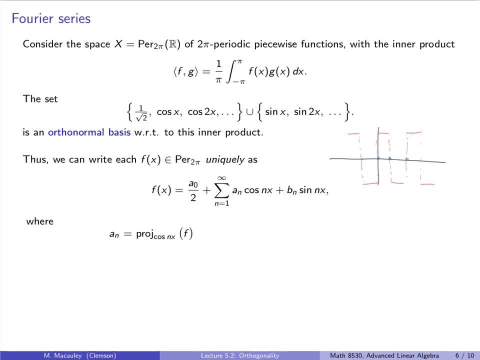 So that again, is a detail that I'm not too worried about. But what I want to focus on is that we have formulas for these a? n's and b? n's. These are just projections of f onto the cosine of n x direction. 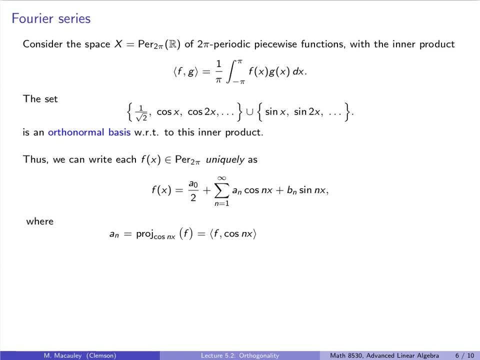 In other words, it's the inner product of f and cosine of n- x. and here is an explicit formula for that coefficient: a n. Similarly, b n is the projection, it's the magnitude of f in the sine of n- x direction. 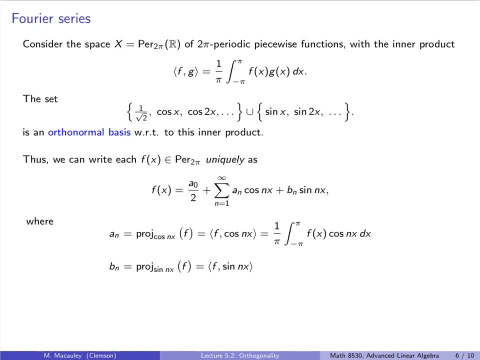 and that's a projection which is the inner product of f with sine of n, x, and that is- here's a formula for that- the integral of f, sine of x, n, x from over one complete cycle divided by pi. Finally, here is that remark. 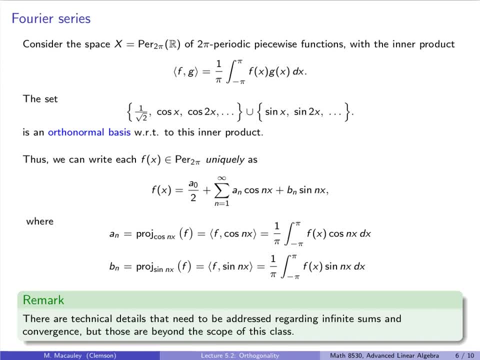 spelled out once more. There are technical details that need to be addressed regarding the use of infinite sums and convergence, but these are beyond the scope of this class and I won't go into details. Finally, I want to say a couple more things. 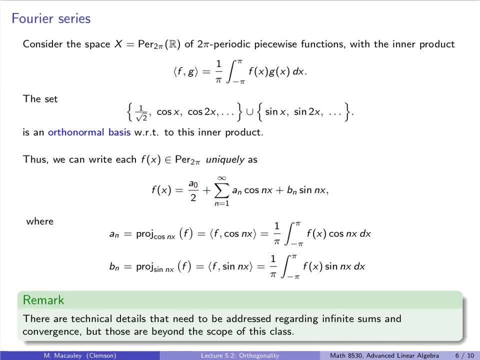 First of all, a naught over two. You know why are we using a two instead of a root two or just a naught? There's a number of ways you could justify this that I won't get into, but one nice explanation. 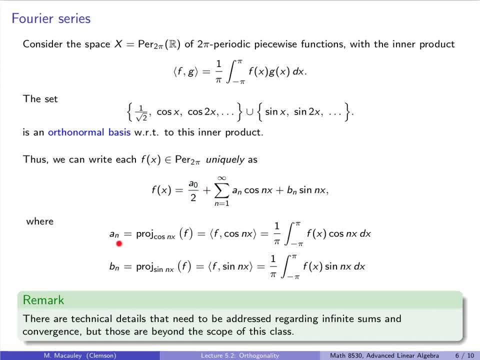 is that this allows the formula for a n to also hold, for n equals zero. So to compute a naught, just plug in zero- cosine of zero is one and compute this integral. I also want to tie this back to differential equations. 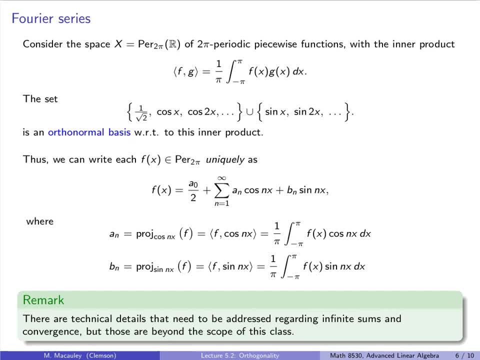 So it is. I said before that my examples would involve differential equations, and this doesn't seem like it does, but here's the connection. So if you have a, say, a vibrating string, and you pluck it in the middle, so these endpoints are held fixed. 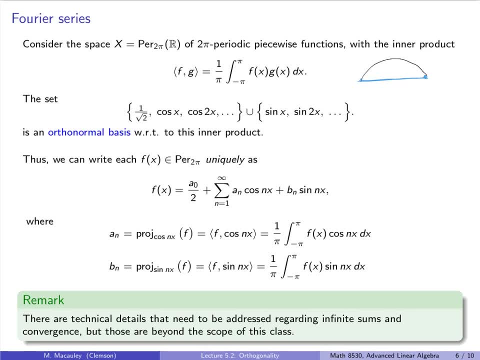 then you can get waves that look like this. You can get waves basically sine or cosine waves. All right, I guess in this case it's sine waves, And these are solutions to a partial differential equation that ut equals c squared uxx. 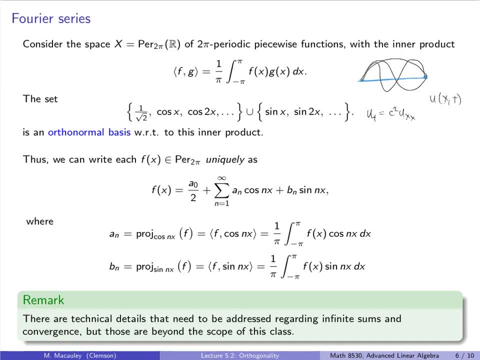 where u is a function of x and t. And when you solve this you basically break up the time and the spatial components separately. and the spatial components, you end up getting y double prime equals negative lambda y And the, and where y is two pi periodic. 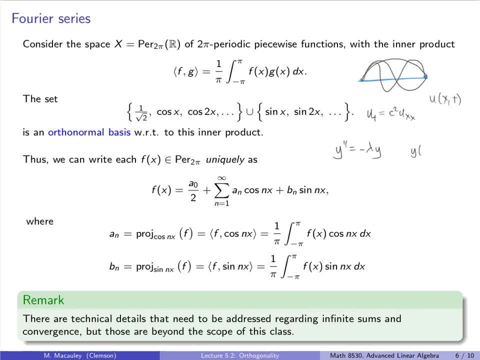 If this is length pi, otherwise it could be something else. So y of x plus two pi plus two pi equals y of x. So solutions to this equation are sines and cosines, and they are precisely at any sine and cosine of this form. 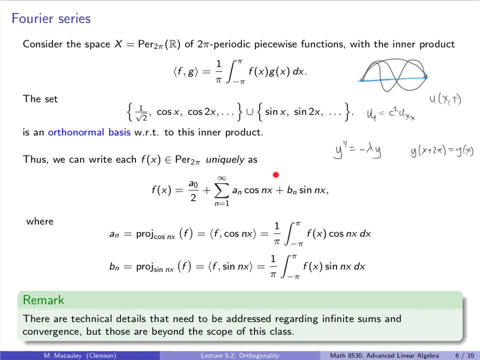 So any solution to this is going to be a Fourier series like this, And even if our initial position of the of the string is is something that's maybe, like I don't know, a triangle wave like this, we can extend this to be periodic. 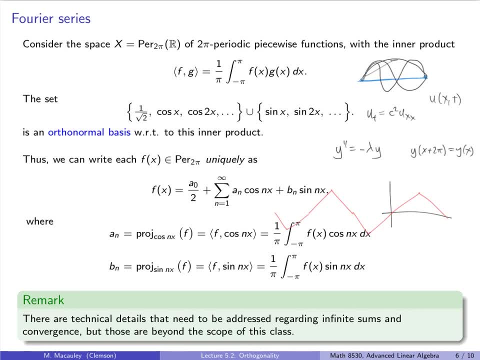 And and physically you can definitely pluck a string. you can start a string in this position and just let go, and there still will be a wave. So even at a function like this, you can write using sine and cosine waves. 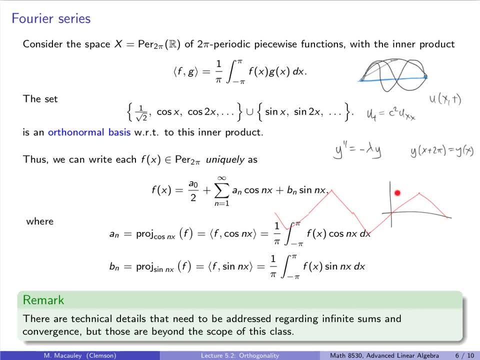 And that's a remarkable fact, because you know these are smooth and this is not. So this, this whole setup of Fourier series, the fact that you can write any periodic function using sines and cosines- again something that an audio engineer 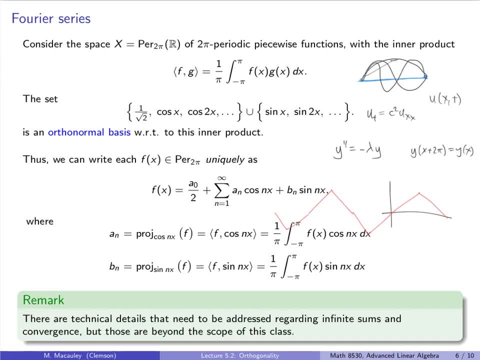 a musician. it's obvious, it's a sound wave. but linear algebra and the theory behind it of vector spaces and inner product spaces not only guarantees that, but it tells us, it gives us a formula for how to compute these coefficients. 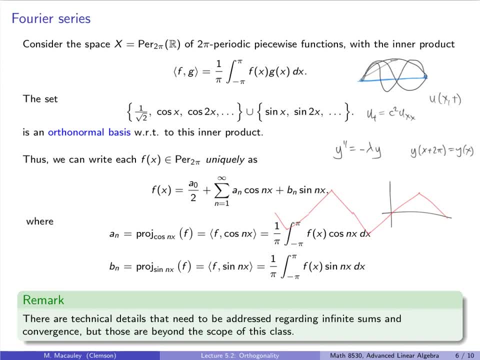 how to find these a? n's and b? n's. And the theory really is no different than how we find the coefficients of this v, which is four e one plus three e two that we did earlier. What is four? Four is the inner product of v onto e one. 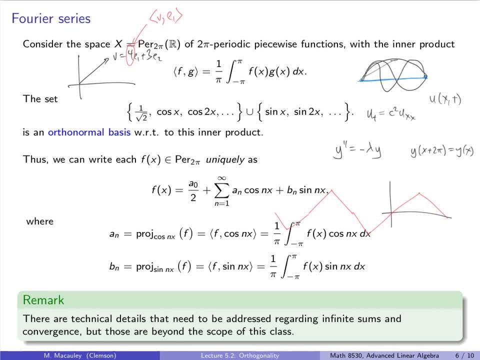 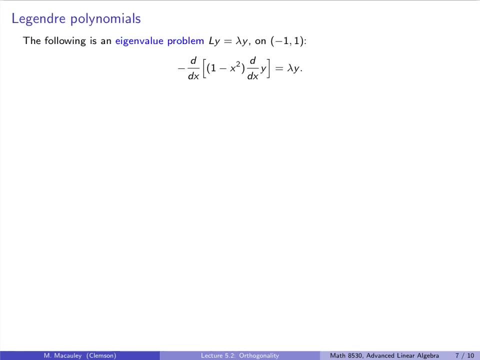 So that's exactly what this is saying here, So it's a really powerful theory that has some really neat results for actual applied problems in science and engineering. And this is really just the beginning. It gets better. Fourier series are a special case of solutions to what are called 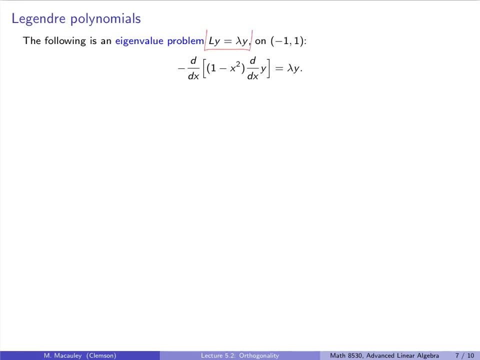 Stroumblouville problems, which are differential equations of the form l. y equals lambda y, where l is a second order differential equation. Here is one such example. I won't get into the details of this. So this is for functions defined on negative one to one. 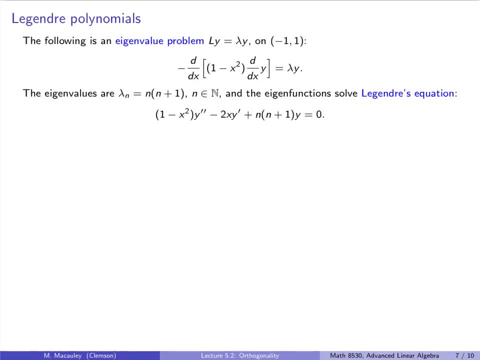 The eigenvalues of this differential operator end up being well, there's infinitely many of them, and they're of the form n times n plus one for positive n, And the eigenvectors, or we call them eigenfunctions, turn out to solve Legendre's equation. 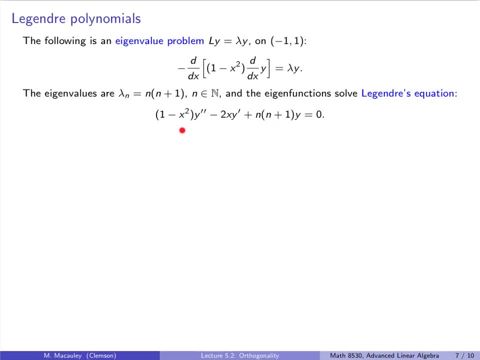 which is a differential equation like this, And this comes up when you want to solve the heat or the wave equation in spherical coordinates For each n. this equation has a two-dimensional solution- space- and one of those is going to be a polynomial. 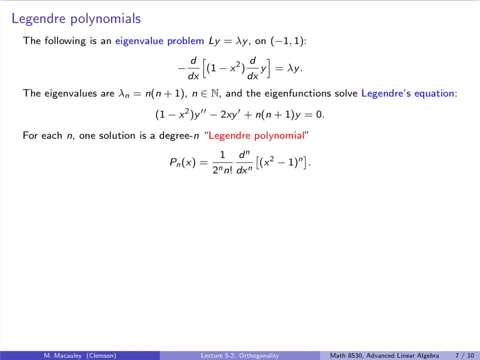 The other one is going to be an infinite power series, And if you take a class in differential equations and you study the power series method, you can learn how to solve them. Now this polynomial doesn't have a nice closed form solution, but it can be defined implicitly like this: 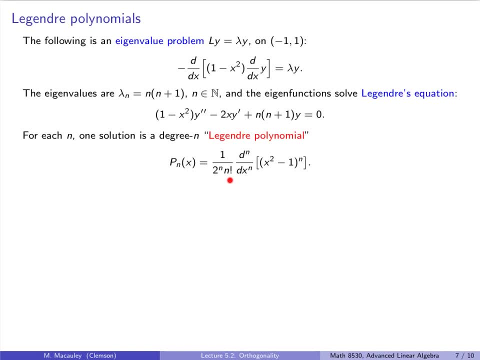 Now it's not clear what it looks like, what this thing is, but this is one way to characterize it And it's a fundamental result of Stroum-Louisville theory that any such equation is going to have eigenfunctions that are orthogonal. 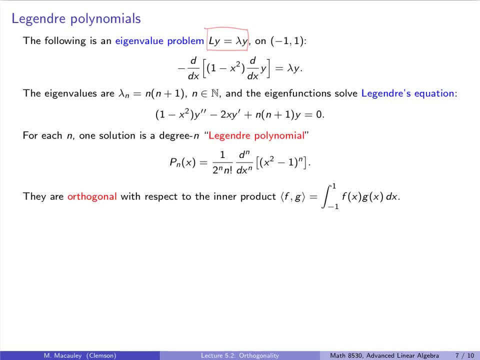 with respect to a certain inner product. In this case it's just f of x times g of x over the interval. So it's a lot like what we saw for Fourier series. but we don't really need to normalize it. There's no reason to. 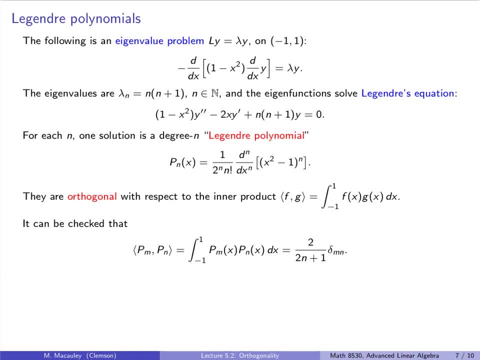 It can be checked that if you take these Legendre polynomials and you compute their inner product, which here's the definition, that they are zero for n and m being different, That's guaranteed by orthogonality. So if m and n are the same, 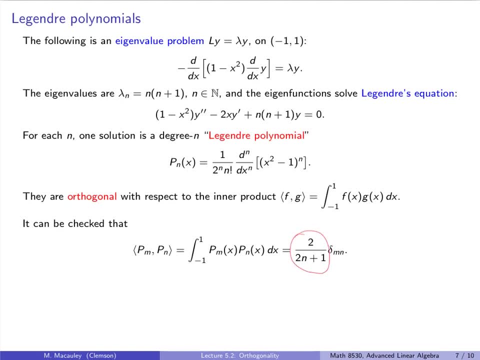 then we don't get 1.. They're not orthonormal, but we get 2 over 2n plus 1.. Now we could normalize them to make them orthonormal, but that's going to mess up this formula and other things. 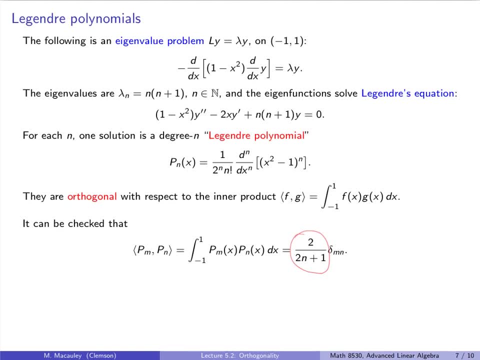 So it's just easier in this case to not normalize and deal with an orthogonal basis instead of an orthonormal basis By orthogonality and the fact that these aren't just orthogonal but an orthogonal basis- every function f that's continuous on this domain. 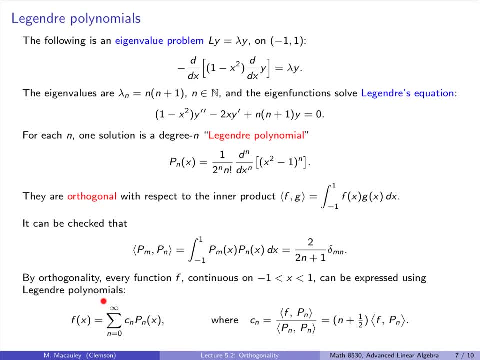 can be expressed using Legendre polynomials. So think of this like a generalized Fourier series. Instead of using sines and cosines, we use these polynomials like this and linear algebra and inner product spaces. The theory gives us a formula for the coefficients: cn. 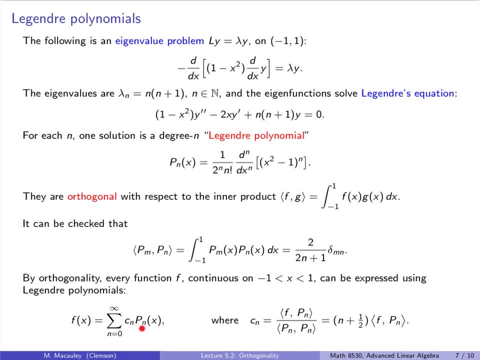 It's just the projection of f onto the nth basis vector, So f dot pn over pn dot pn, And if you simplify that, that's just n plus 1 half times the inner product of f with pn, And this we have a formula for right here. 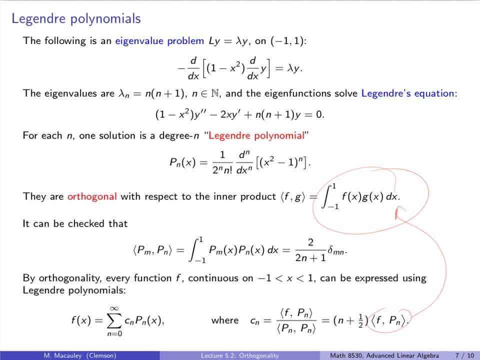 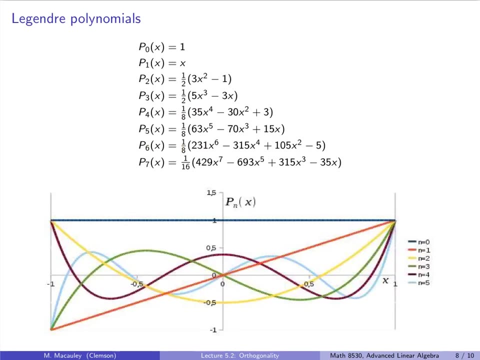 So, once again, the power of linear algebra allows us to write arbitrary functions on negative 1 to 1 using Legendre polynomials. And here is an example of the first eight Legendre polynomials, both what they are algebraically and what they look like graphically. 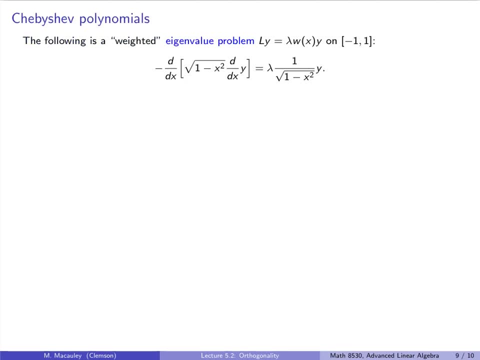 Finally, our last example is also a Strum-Louisville problem, And you can think of it like a generalized eigenvalue problem, because you have this: it's not ly equals lambda y anymore, but you've got this weight here, And if you want to know more about this, 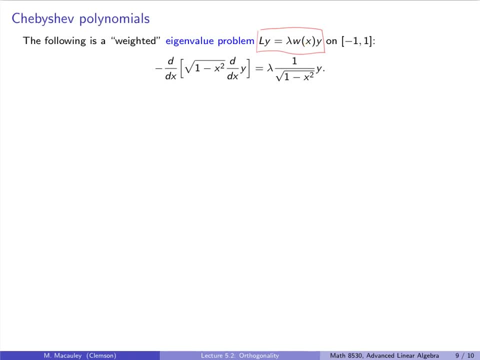 take a course on Fourier analysis, a graduate-level course, or functional analysis, to motivate why this thing comes here. But in this particular case that w is this: 1 over root, 1 minus x squared. So this is Chebyshev's equation. 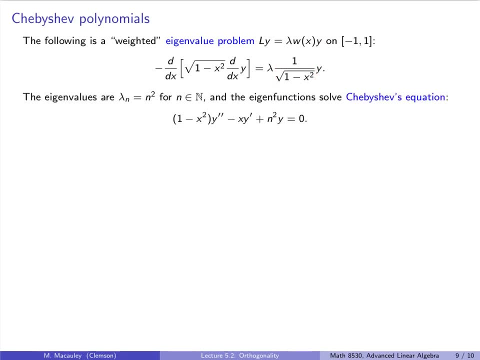 It comes up a lot in numerical analysis techniques, And the eigenvalues for this are n, squared for any positive integer, n, And the corresponding eigenfunctions solve Chebyshev's differential equation, which is well, it's basically what you get from this. 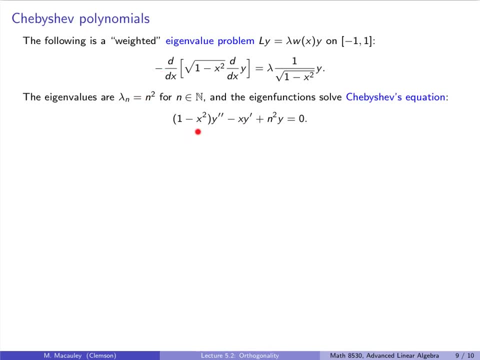 by just plugging this into lambda and simplifying, But it looks like this. Once again, you can solve this using the power series method. You get two linearly independent solutions, And one of those is going to be a polynomial. It's called a Chebyshev polynomial. 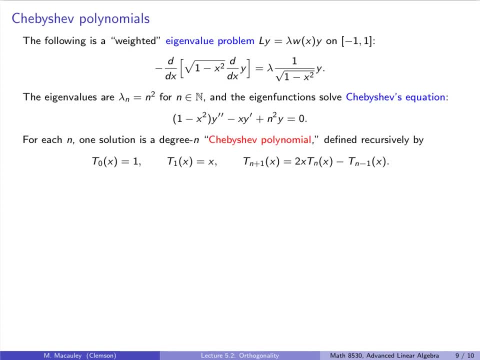 And for this one it's easiest to define it recursively. So the zeroth degree 1 is 1.. The first degree 1 is x, And then you have this recurrence relation: The n plus first 1 is 2x Tn minus Tn minus 1 of x. 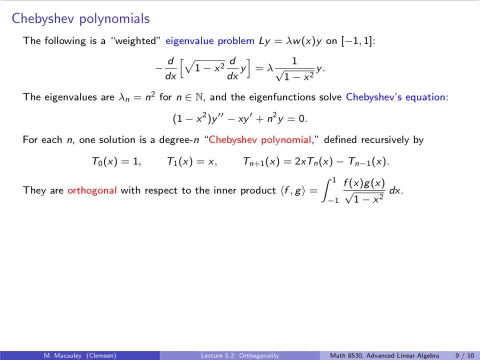 Bystrom-Liouville theory these polynomials are orthogonal with respect to the inner product, So it's going to be like the last one. but we have to multiply by this weighted function w of x here, So the integral of f of x, g of x. 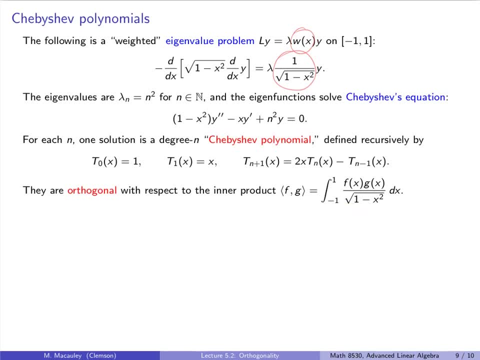 divided by root, 1 minus x squared dx. And it can be checked that if you take two Chebyshev polynomials and you compute this integral, well, if n and m are different, then you're going to get 0.. So that's why this delta is here. 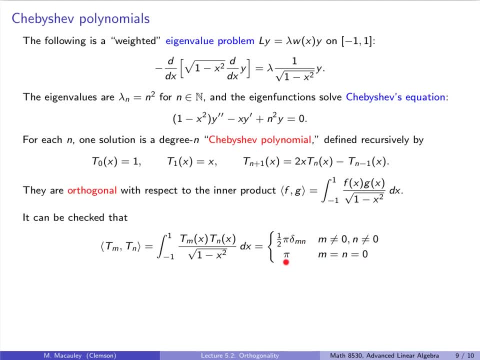 But if they're the same, well, if they're both 0, you actually get pi, But if they're the same and non-zero, then you get 1 half pi. So they're not quite orthogonal. They could be normalized. 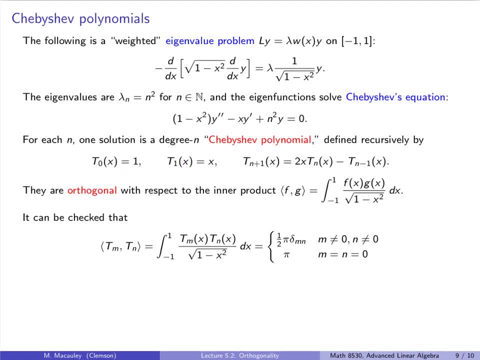 but if you normalize them that's going to mess up this recurrence relation. So it's just easier to deal with an orthogonal basis rather than an orthonormal basis. But by orthogonality every function f, that's continuous on negative 1 to 1,. 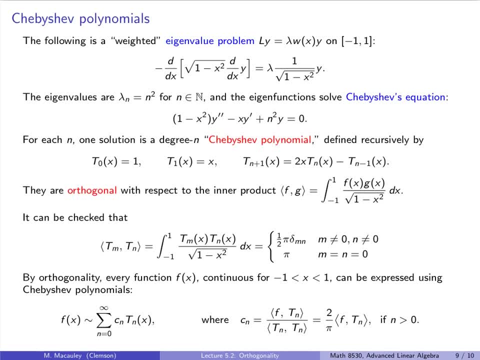 can be expressed using Chebyshev polynomials And we can probably weaken this continuous a little bit, but it's easier just to make it continuous. So it can be expressed as a linear combination of Chebyshev polynomials And, once again, this Cn. 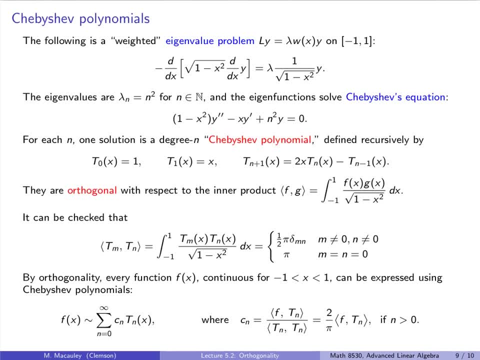 is just the projection of f onto the nth basis vector, Tn, And if you use this formula, that's just 2 over pi times the inner product of f with Tn, which is, of course this is given by an integral. 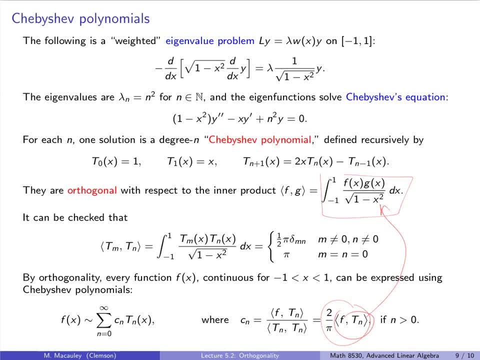 or that part's given by this integral right here. Now one little detail. you may have noticed that I, instead of using equals, I used this little similarity. So, technically, this is one of those details that I'm not going to get into. 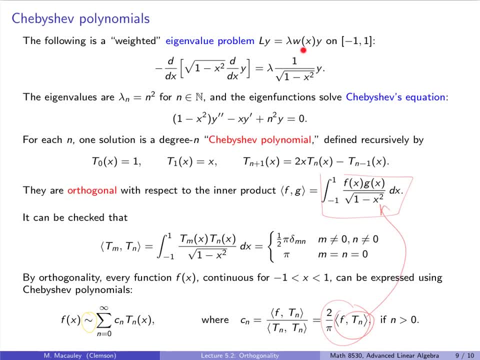 There's a strange norm because of this weighted function. So there's a diff. When I say converge, when I say f, Saying f equals this, I really mean f converges to this. You know, you might look at it at a picture. 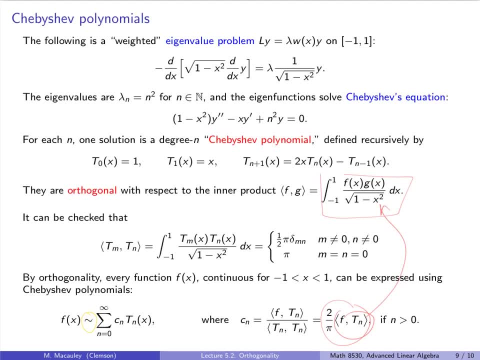 and say: well, that doesn't look like it's converging very fast, And that's because it's the difference of converging pointwise versus converging in norm, especially when we have a norm that involves a weighted function. So this is some functional analysis.